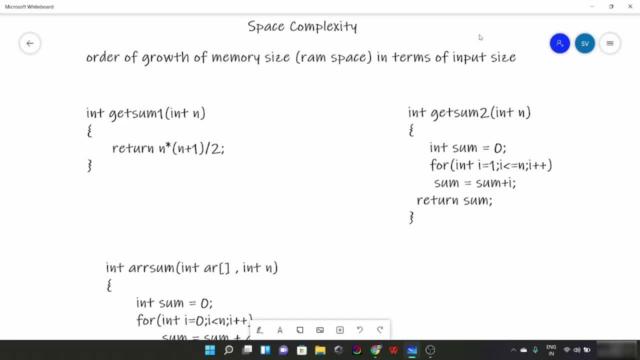 Hello everyone. So today we are going to learn about space complexity. So space complexity is order of growth of memory size, or RAM space amount taken in terms of input size. So, as you can see, it is very similar to time complexity, which is, as we know, order of growth of time. 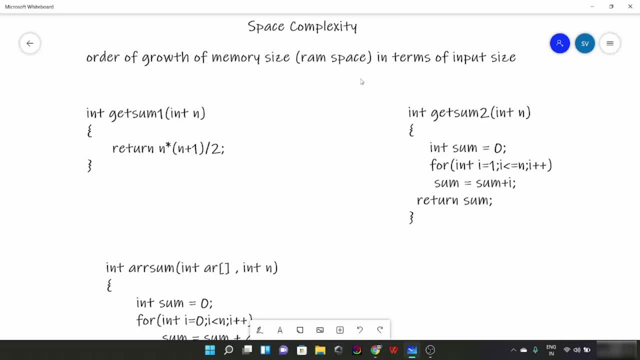 taken in terms of input size, But here, instead of time taken, it's memory taken or RAM amount taken. Now let's see few examples to understand better about space complexity. So let's see this function first. So in this function we are determining sum of first and natural. 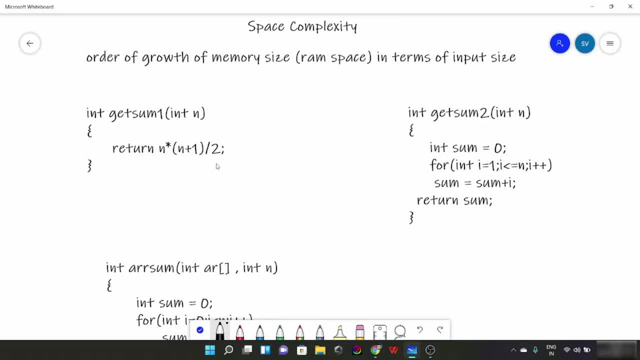 numbers, And here we are using the direct formula, And I'm assuming you must be knowing about this formula. All right, Okay, So can you tell me the number of weights? Yes, The number of variables? here The number of variable is only 1, n. Right, And we can see. 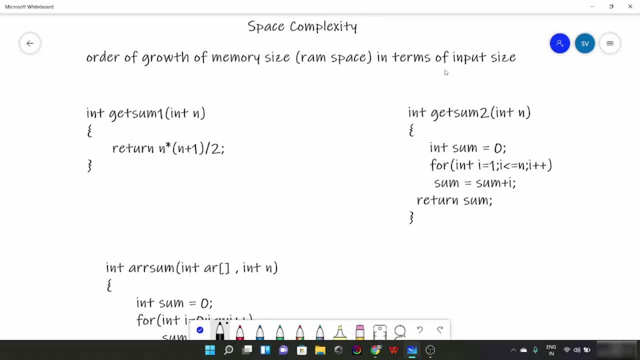 that space complexity is, you know, order of growth in terms of input size. All right. So suppose if n is 100, then the number of variables would be still 1. Right. And suppose n is 1000, the number of variables would still be 1. So number of variables is not depending on. 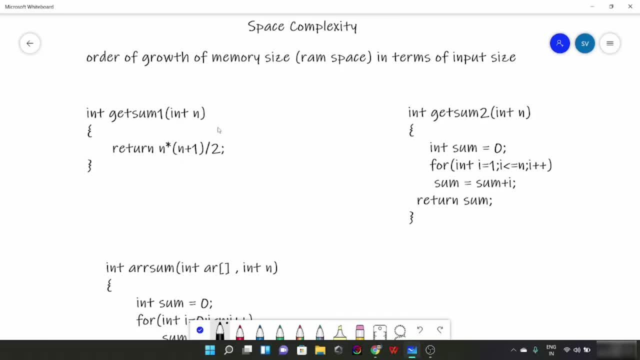 input size. So we can say that space taken by this function is constant. So we can write space complexity as theta 1.. Right, Okay, Let me tell you that as long as number of variables are constant- Okay, Meaning it's not array or list of variables- then the space complexity would remain. 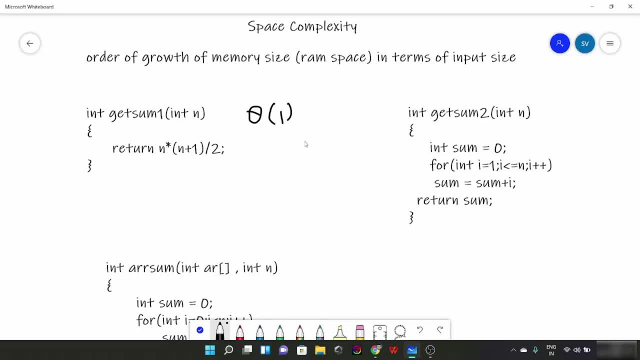 constant, All right. So once you can see that space complexity here is theta of 1 or constant space taken, All right. Now let's come to this example, this function. So what this function is doing? it is also computing some of first and natural numbers, But here we are adding numbers, one by 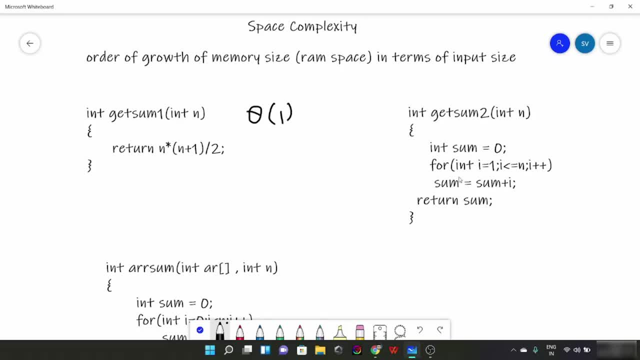 one in this function. All right, As you can see, in this function, as this loop, All right, Now count the number of variables here. All right, you know: n, first variable, sum, second variable and i, third variable. now, if i ask, if we change n, 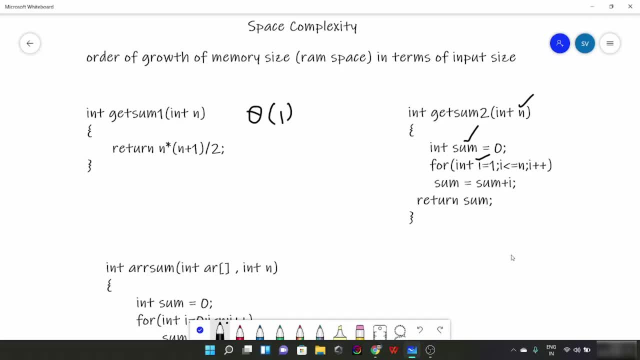 suppose let's take n 3, then the number of variables would be 3. if n is, suppose, 100, the number of variables would still be 3. and sum i, if n is 10, 000, then the number of variables would still be 3. so we can see that number of variables is not depending on input size. so we can say that the 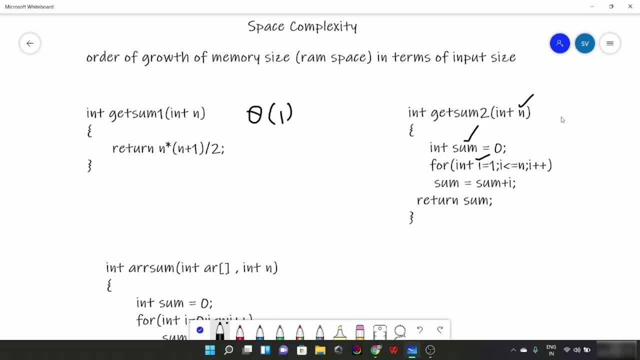 size taken by this function is constant. so you can say: space complexity of this function is theta 1 or constant space. all right, as i told you before that if the number of variables are constant, irrespective of changing our input size, the space complexity would be constant. right, all right. now let's come to this example. all right, this is a very important example. 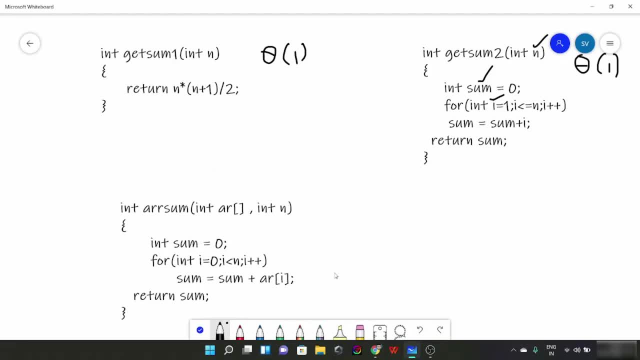 so here what we are doing. we are having a function which takes our parameters as array, an array and its size, array size, all right. and then we find the sum of all the elements of array through this loop and then we return the sum. all right, simple function. now tell me the number of variables here. 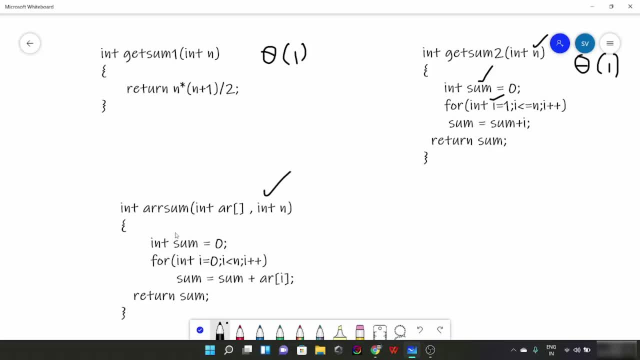 so, uh, one variable n, one variable sum and one variable i, only three variables. and, and one more important thing, number of elements present in this container, which is our array container. right, this will also contain elements, so this will also like contain variables, which will have elements of this container. all right. now, suppose n is 100, then how many variables? 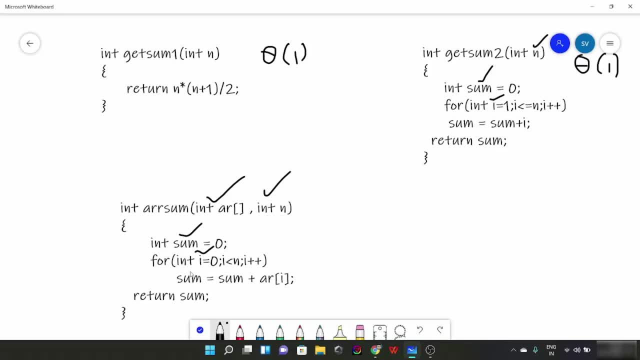 would be there one variable, second variable, third variable, plus 100 more variables, the elements of our array. right, if n is thousand, then elements would be what one, two, three plus thousand elements was. n is, you know, input size of array. so array would contain thousand elements. so we can see that number of elements here. 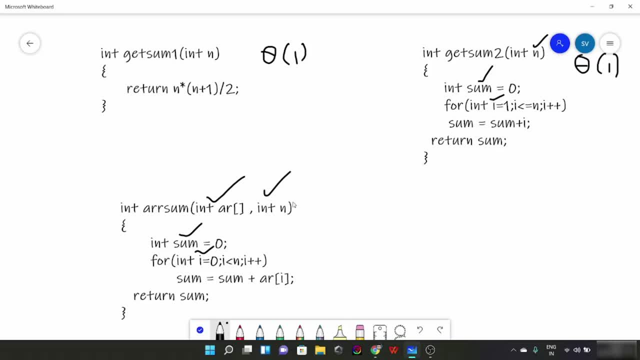 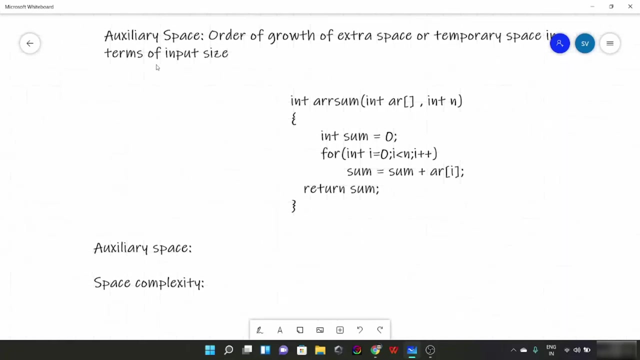 is direct are directly proportional to input size, which is our n. so you can say that space complexity here is theta n, right? so this is how we calculate space complexity. i hope this gets clear to you all. right now let's talk about one more important term called auxiliary space. auxiliary space is order. 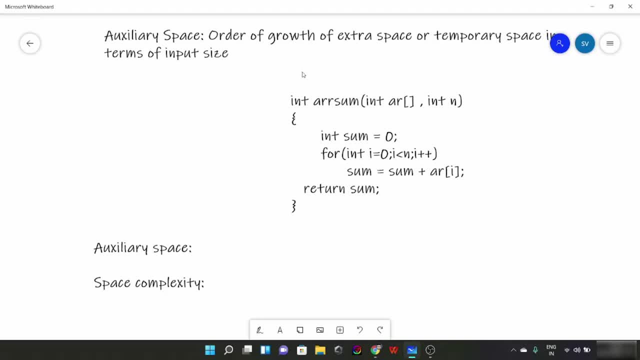 of growth of extra space or temporary space in terms of input size, all right. by extra space, i mean the space created a memory other than input or output. all right. so let's see this example. so here this is the same function as we saw before. is so we want to remember to say that more previously i talked about geometry. 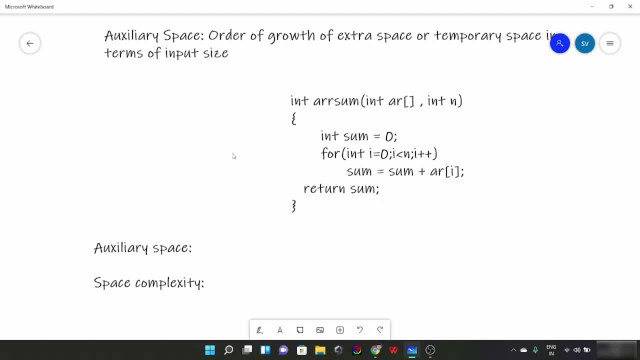 and volume. today this is generate strings. Finished. so first let us go to ok and to manually add the other function which is your function. doing this, we just run deduct Q and vice versa. ok, so so this is change written regulations to the space. complexity here. so this function will still the same. right here, besides the $ perform parameter and then the $ of this function then does not calculate. 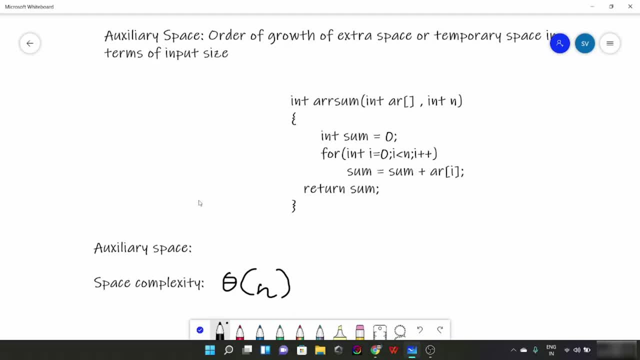 So what did we say about auxiliary space? That it is extra space created which is not related to input or output. Alright, So, as you can see, in this function it only takes array, this array as input, and no extra array is used for computation. 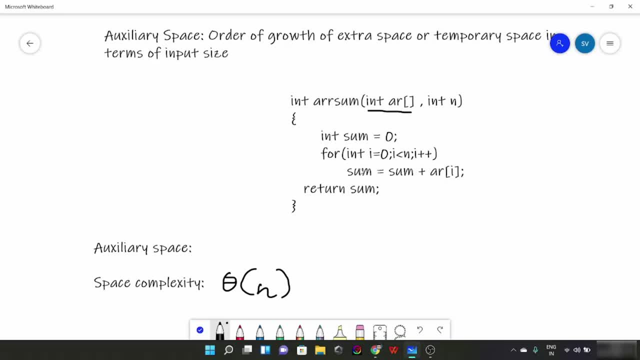 The only auxiliary space here is the declaration or space taken by these variables sum and i. Alright, And if we change the size, or if we change the input size, which I mean n, then still the number of variables would remain constant. Hence auxiliary space would still be constant, which is theta of 1.. 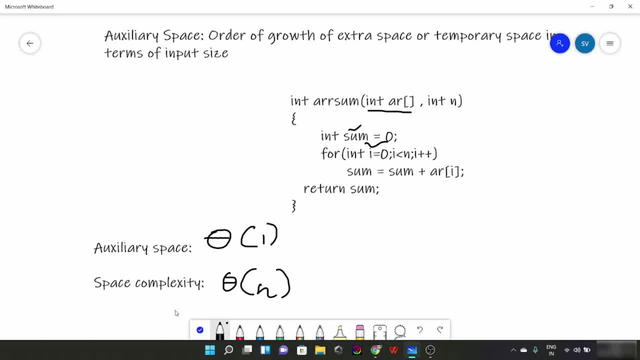 Right. So I hope this is clear to you, that what is auxiliary space Right Now? if I ask you like, if we have to compare two functions to find the efficiency, then what would be the deciding criteria? So a direct answer, it would be: 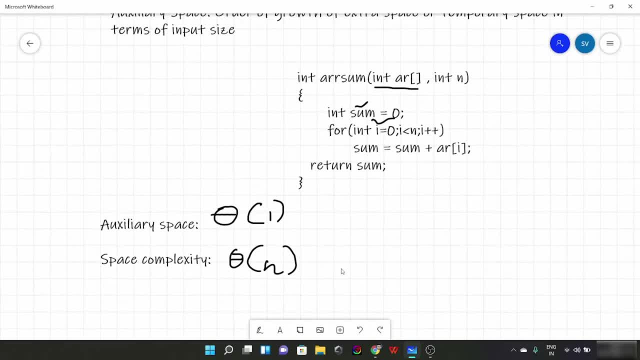 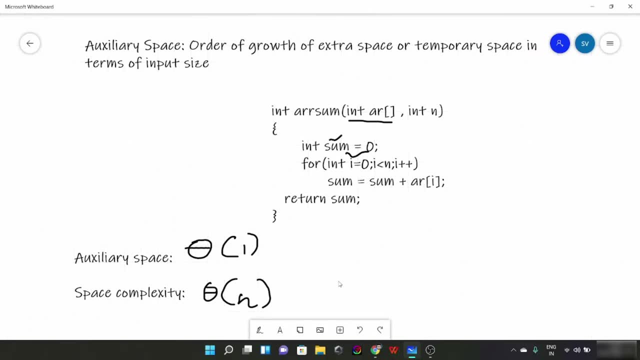 Auxiliary space. Alright. Now you might be wondering why. Alright? Now let me tell you about it. Suppose, if you talk about array problems, list problems or any problems which use input containers, then they are going to use theta n space for input. 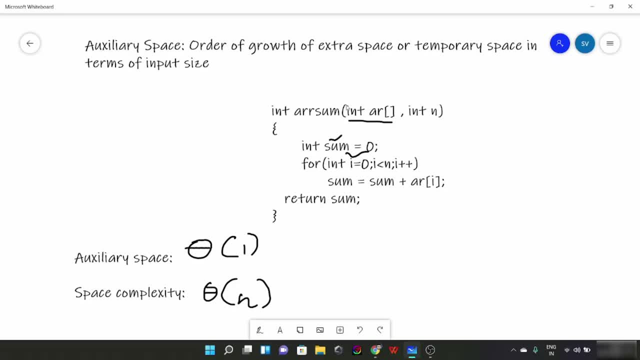 Right For passing array into their perimeter, like in this function, Right? So space complexity would be theta n. Right? So if suppose, if I use an extra array here, of suppose a Right Of size n, Okay, So the time complexity array, the space complexity, would still remain, you know, theta n. 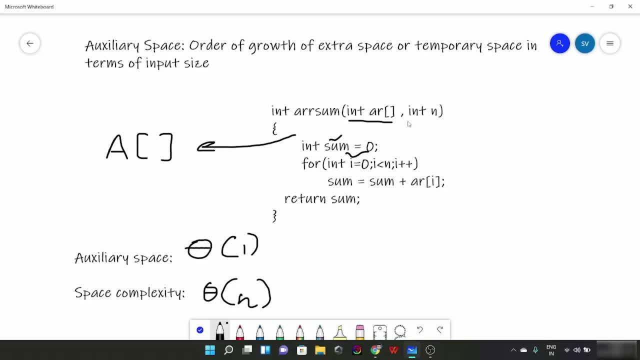 Right, Okay, Okay. So let me tell you what would be the space taken by this one. It would something be c1n, Right? What would be the space taken by this one if there was this function: c2n. 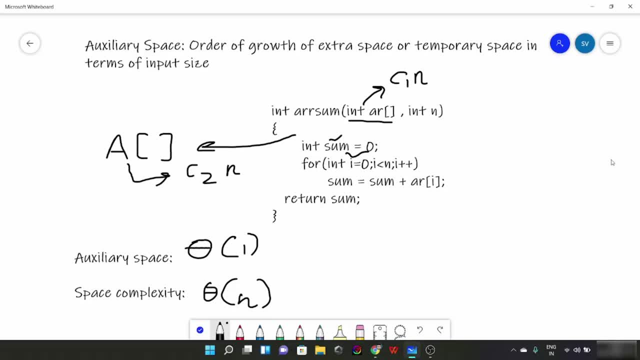 And then there are some variables which would take time, something c3.. So what would be the total space taken, c1n Plus c2n Plus c3.. Right, So we can you know club c1 and c2 and we can say something c4. 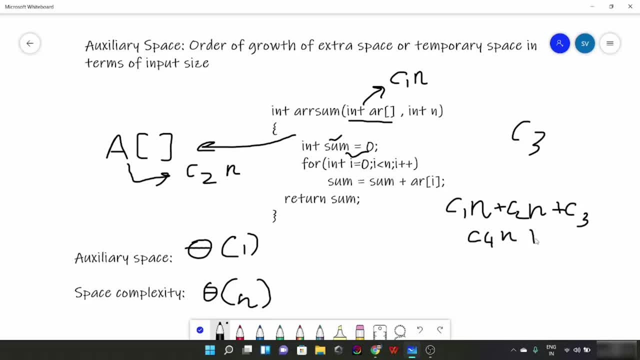 So it would be, you know, c4n Right Plus c3.. Yes, And if we find the order of growth, what would it be? We will ignore the linearity, We will ignore the lower order terms and we will ignore the coefficient of feeding term. 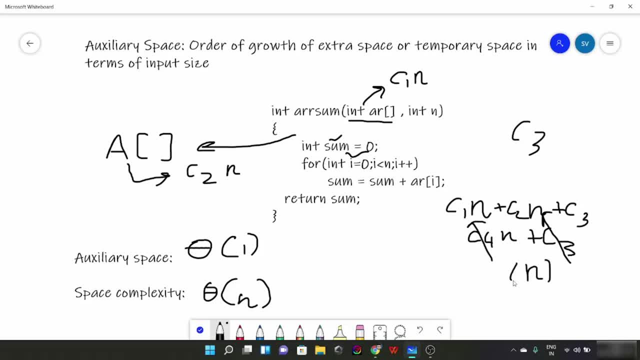 So it would be n right. So this is what I was talking about. If we add this, we will still have the space complexity of theta of n. But what would change here? This auxiliary space, right Auxiliary space, would change here. 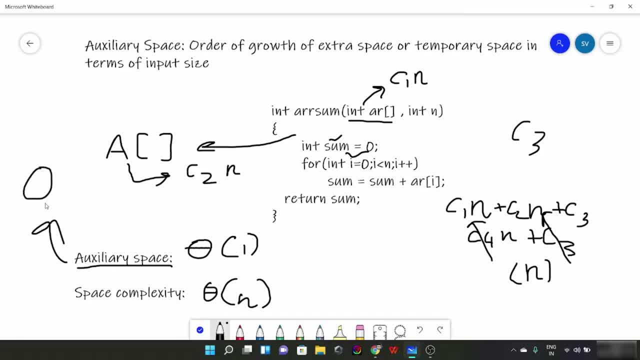 It will then become theta of n right. So this is what I was talking about. We are, you know, more concerned about auxiliary space or extra space taken by the function. All right, So let me tell you about something, about sorting algorithms, which will come later in this series. 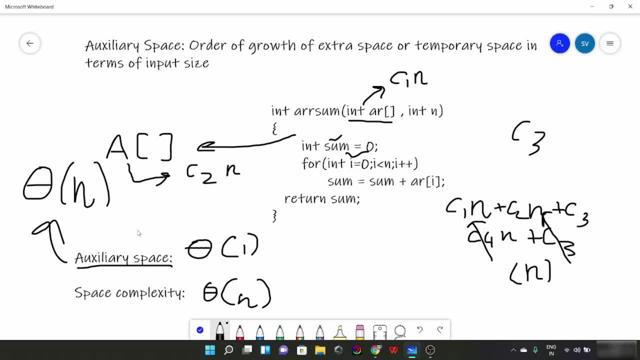 Suppose, if we talk about sorting algorithms such as, you know, bubble sort, quick sort, insertion sort, etc. What they do? They don't take any extra Array to sort the to sort, All right, So their auxiliary space would be theta of 1, right. 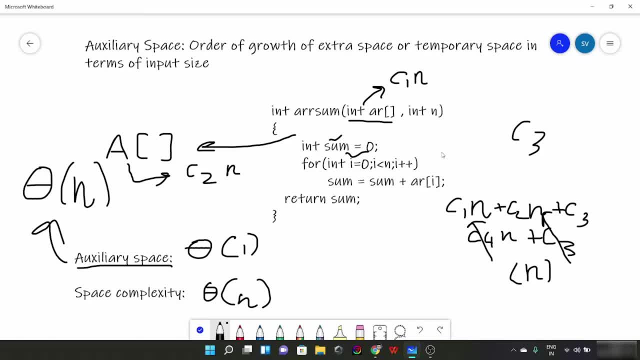 But there are some sorting algorithms, such as merge sort, which requires an extra array to compute the sorting. All right, So its auxiliary space becomes theta of n. Now, in all these sorting algorithms, we have to, We have to pass input array into the functions, right? 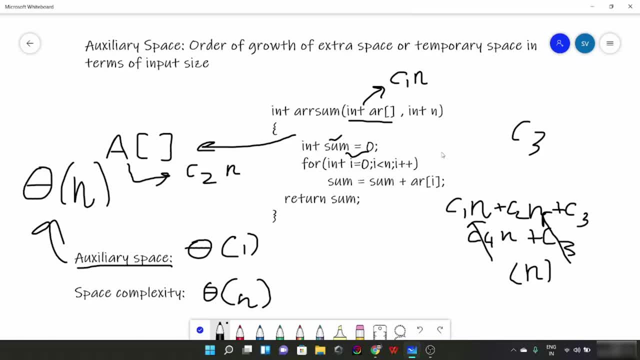 Whether it be bubble sort, quick sort or merge sort. So in every case, the space complexity would be theta of n. All right, So what would be the- you know, the deciding criteria? What would be the deciding criteria then?